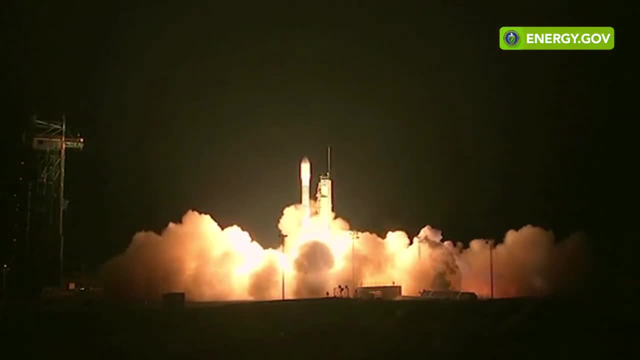 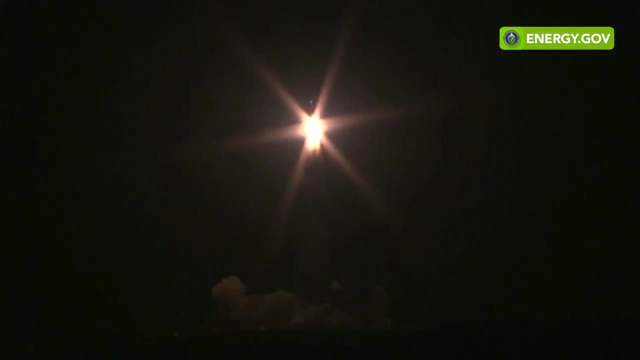 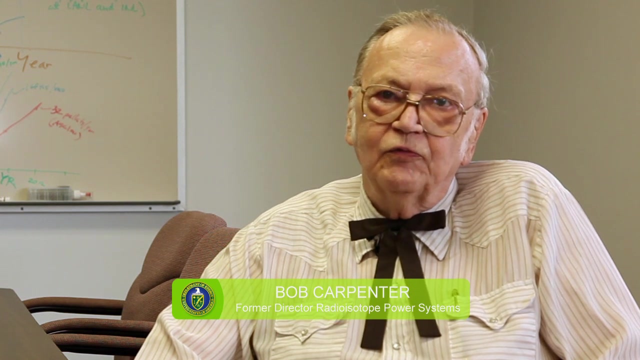 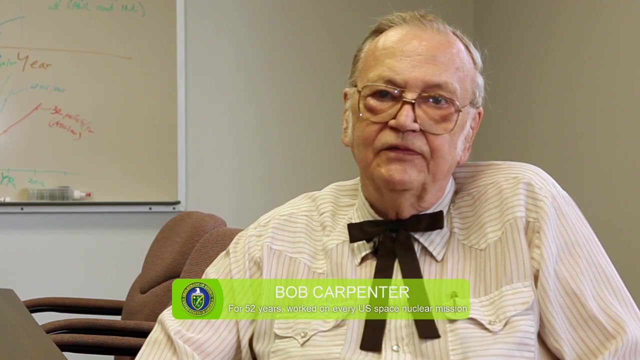 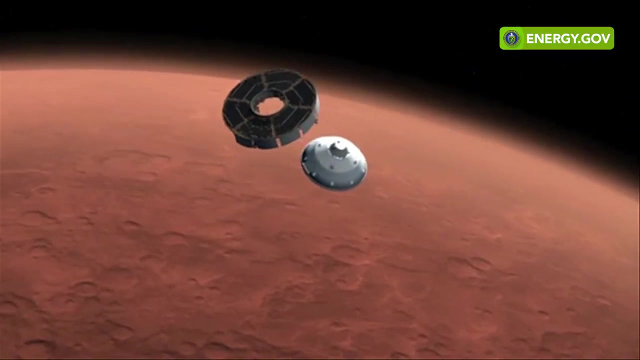 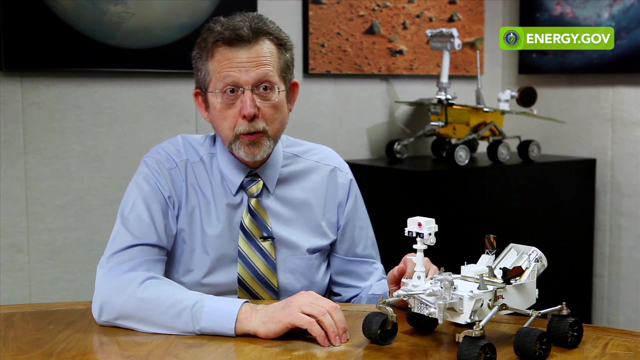 Main engine, start one zero and liftoff. If the US citizen wants the US to stay in a world leadership role in space exploration, you have to have radioisotope power systems. On November 25th, a window opens and it allows us to launch the Mars Science Laboratory. 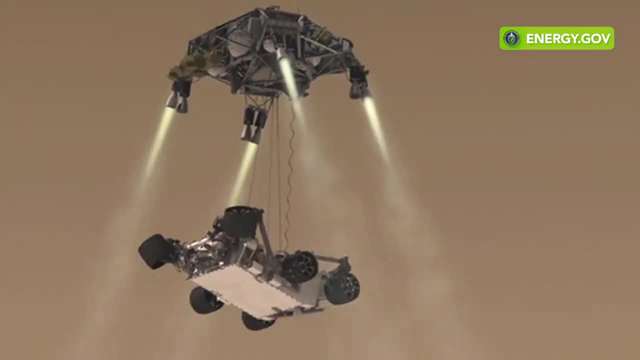 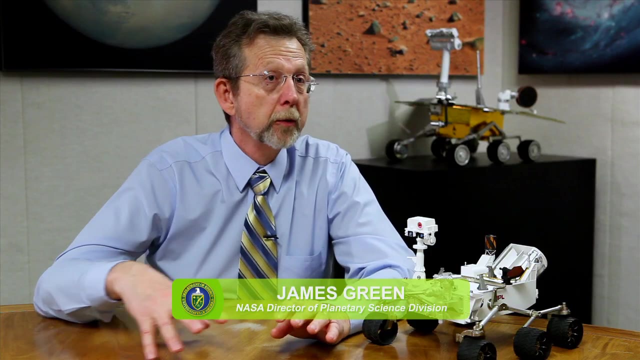 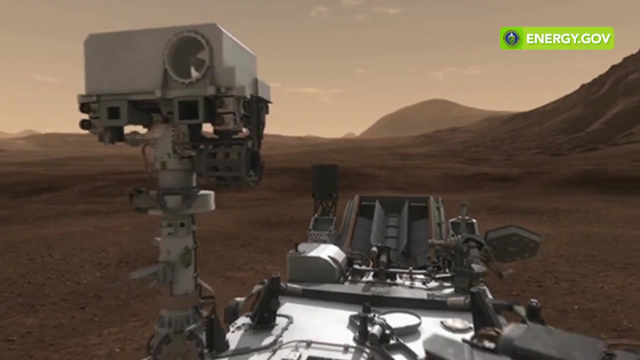 That particular mission will land a rover called Curiosity on the surface of Mars. It uses radioisotope power because it has to be able to operate through the winter, could potentially operate through the night, and it goes into the regions where there are low sunlight conditions. 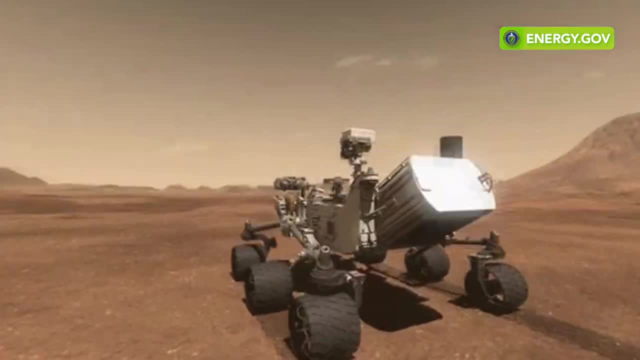 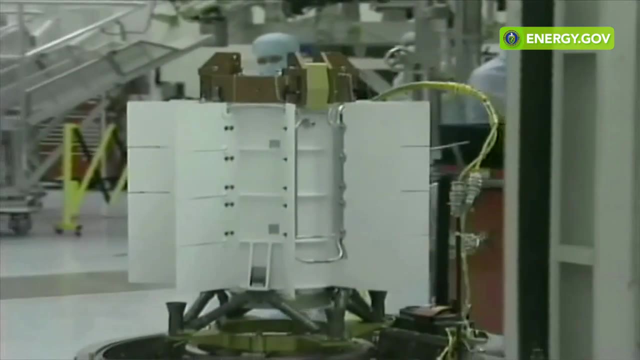 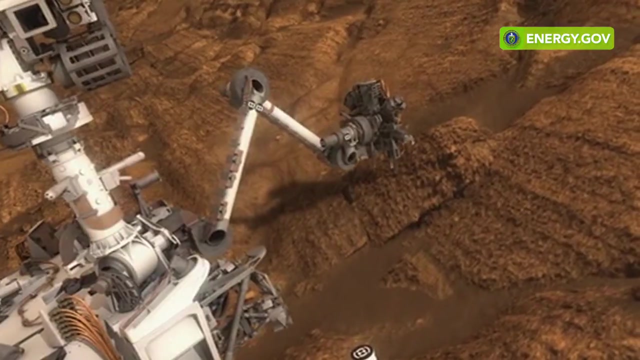 and so it therefore needs its power. It needs its power supply to operate. A radioisotope power system is a kind of nuclear power system which uses the natural decay heat of a radioisotope- or in this case plutonium-238, to generate electricity which can be used by a spacecraft. That's important, because it enables us then to run experiments. charge batteries survive the night. We can use the heat from these systems to keep everything at a particular temperature that allows it to survive, And because of that we have certain missions that we could have never done using traditional solar power. The first nuclear-powered satellite was launched in 1961. It was the Navy's Transit 4A satellite. It was used by the Navy as a predecessor to today's Global Positioning System satellite network. They were first developed under the Atoms for Peace Initiative under President Eisenhower. 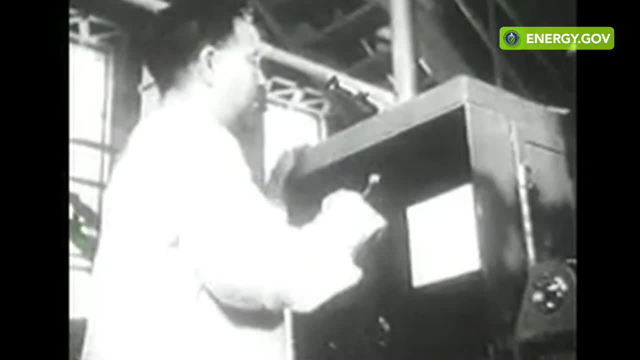 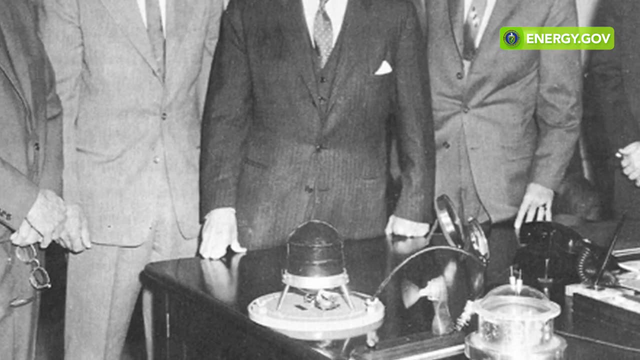 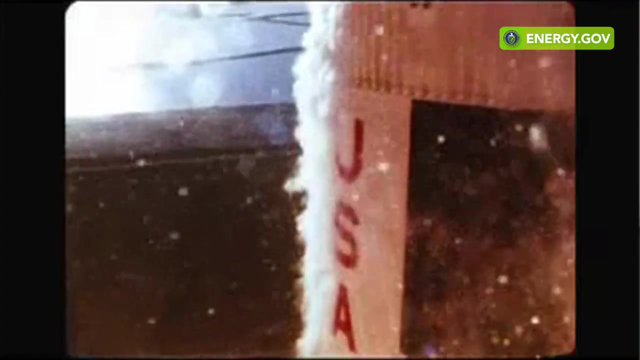 First encourage worldwide investigation into the most effective peacetime uses of fissionable material, And the first public introduction to a radioisotope thermoelectric generator was in President Eisenhower's Oval Office. Since then we've launched over 27 missions using nuclear power systems in outer space. 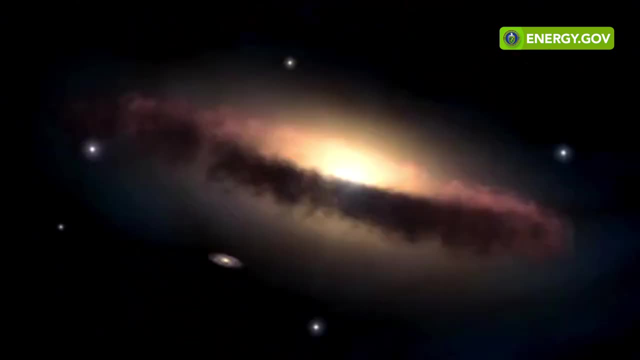 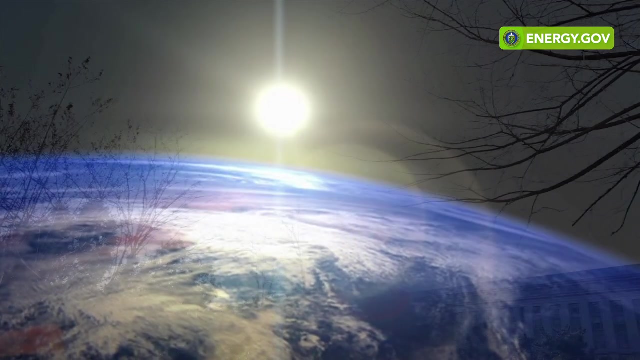 So, then, NASA began using RTGs to enable their deep space exploration for about a decade, And during this time there were some changes back here on Earth. The Energy Research Development Agency became the Department of Energy, And since then the Department of Energy, with NASA, have teamed up to produce. 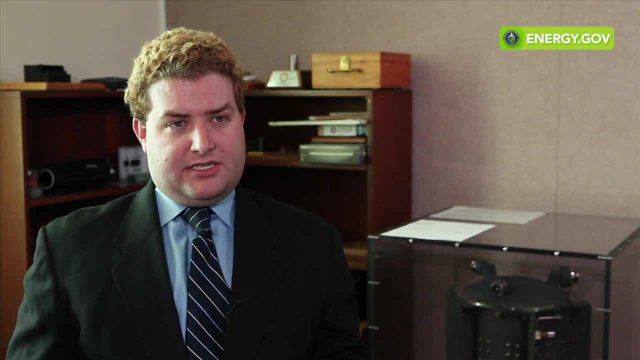 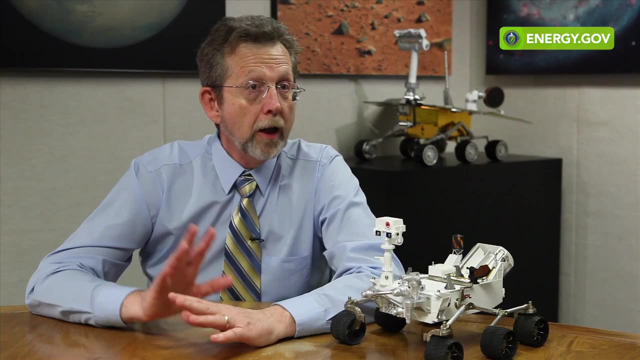 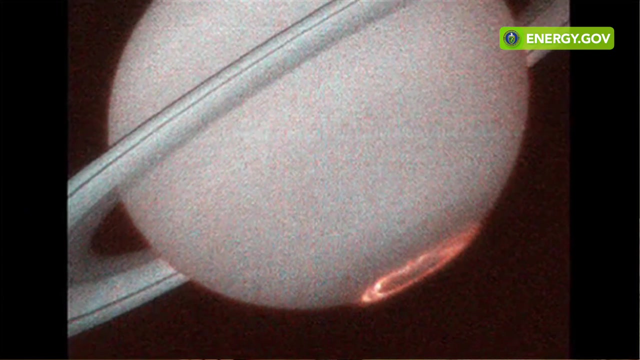 long-lasting, reliable power systems for deep space exploration. We've had generators on the Moon. They've done flybys of Venus, Uranus and Neptune, The Galileo mission to Jupiter. We're currently orbiting Saturn with the Cassini spacecraft.